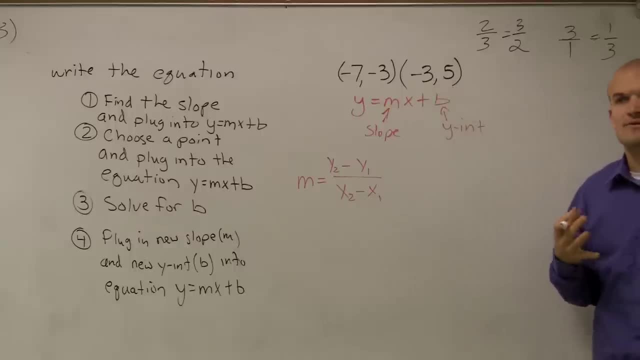 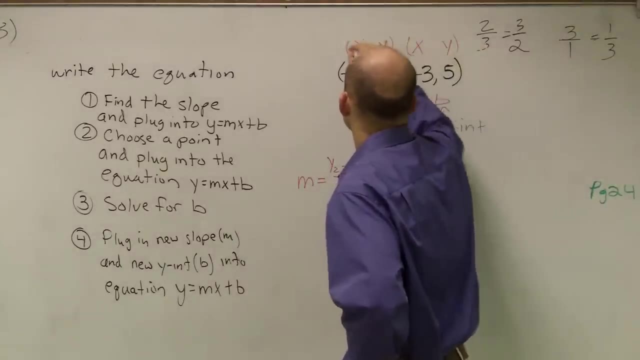 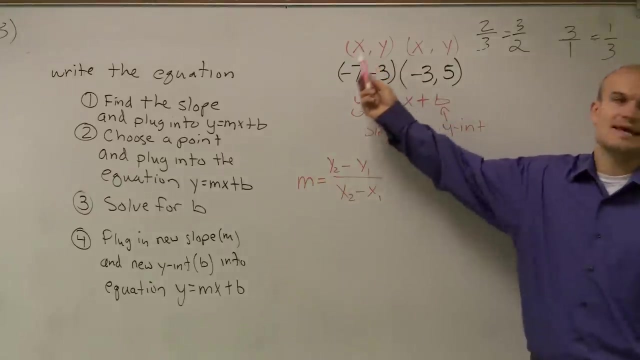 Well, remember, when given two points, we can find what the value. we can label them x and y, right? Remember, every coordinate point on a graph has an x and y coordinate. However, the problem with this is we don't know when I say x, we don't know which x. 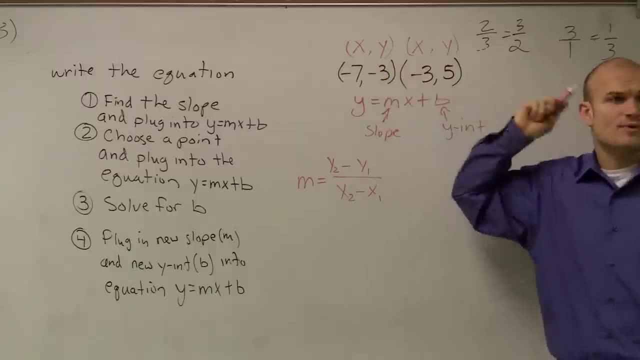 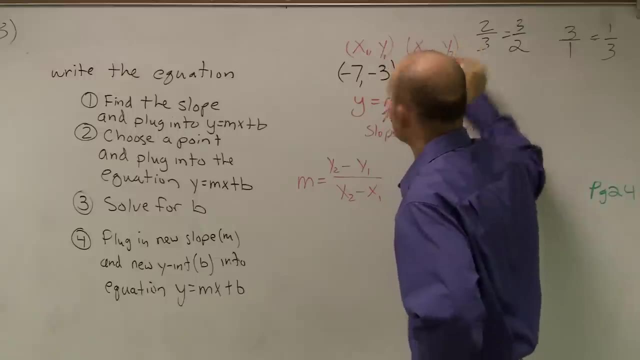 we're talking about. Justin. can you just kind of write on your own paper, please? So we don't know which one we're talking about. So what I'm going to do is I'm going to label this x1 and x2, y1 and y2.. 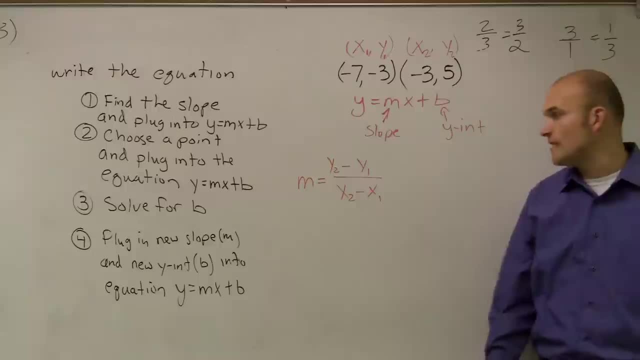 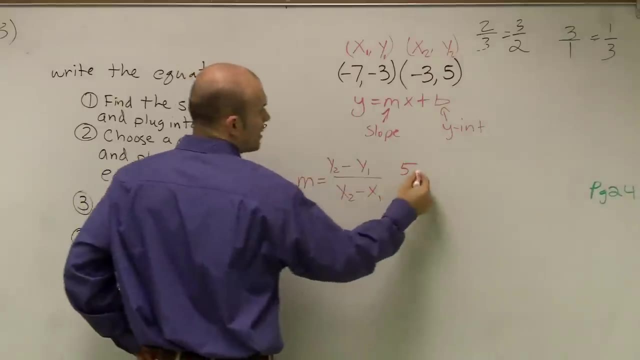 That just helps me distinguish my x and y coordinates. So then, what I'm going to do is I'm going to plug them into my equation to find my slope. So y2 is 5, y1 minus y1, all over x2, which is a negative 3,. 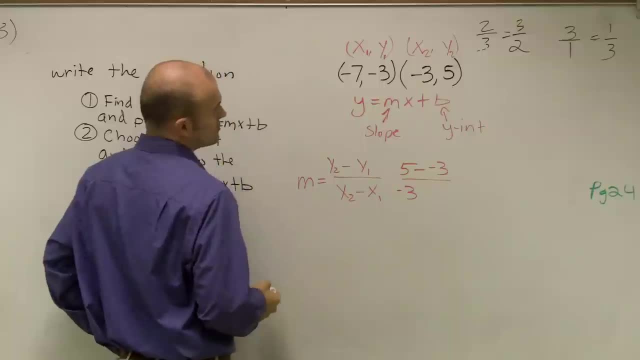 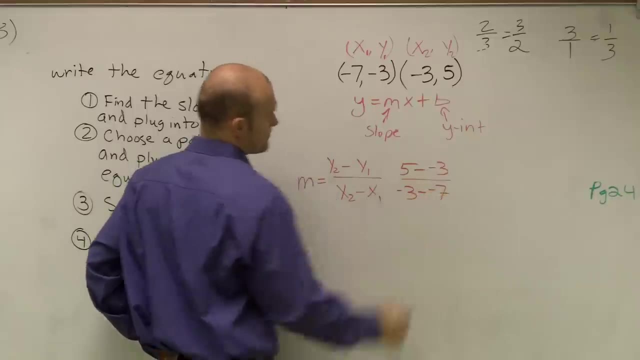 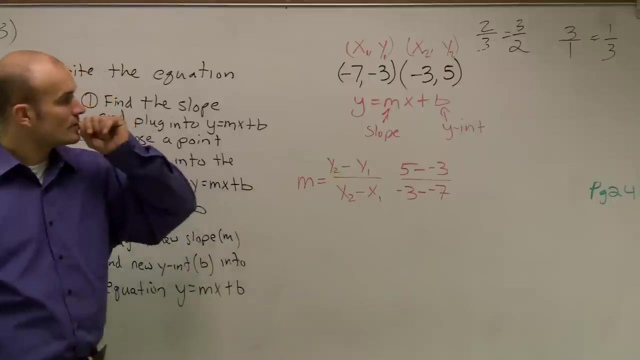 minus minus a negative, 3, minus a negative 7.. Okay, Remember it's your change in y over your change in your x's. So therefore, 5 minus a negative 3, that's a double negative becomes positive, which is 8.. 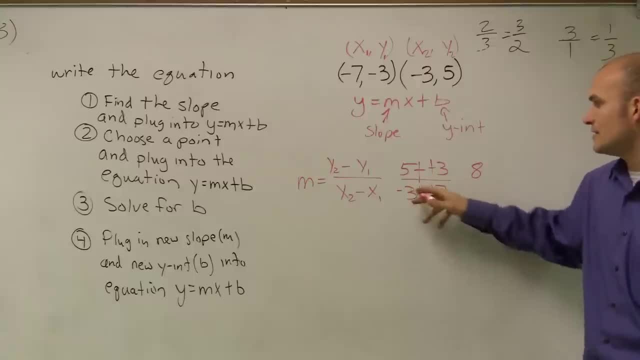 Negative 3 minus a negative 7, again we have a double negative. Negative 3 plus 7 is going to be a positive 4. Therefore, my slope is: 2. Negative 3 minus a negative 7. When you have a number minus a negative number, it's a double negative, so it turns to a positive. 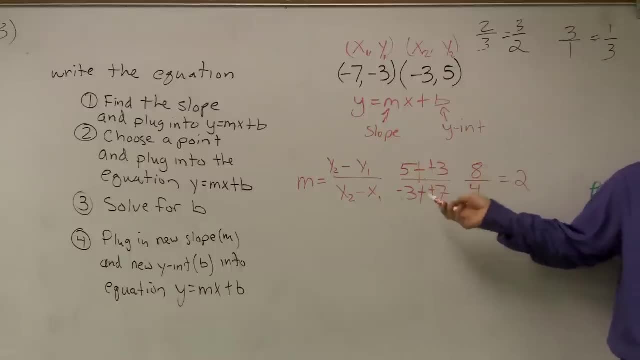 Or it turns to adding, So it's a negative 3, add a 7,, which gives you a 4.. So therefore, Yep, what 8,? 4 goes into 8 two times. That's where I got that. 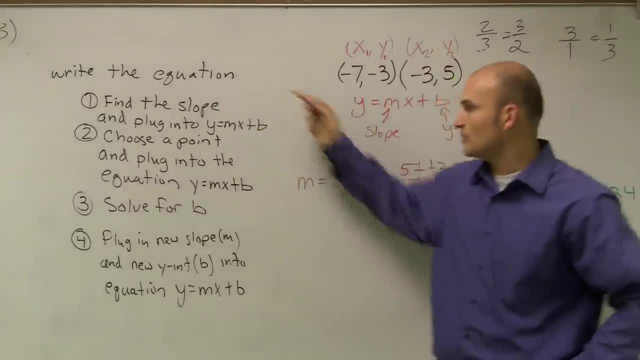 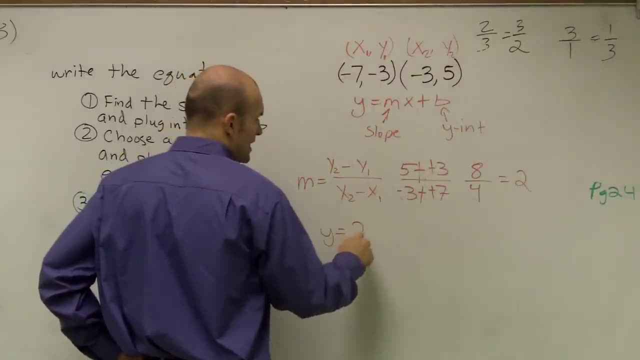 So now What I wrote up there is, I find the slope, which I did, And then I need to plug it into y equals mx plus b. So I say y equals Instead of m, I can say 2x plus b. 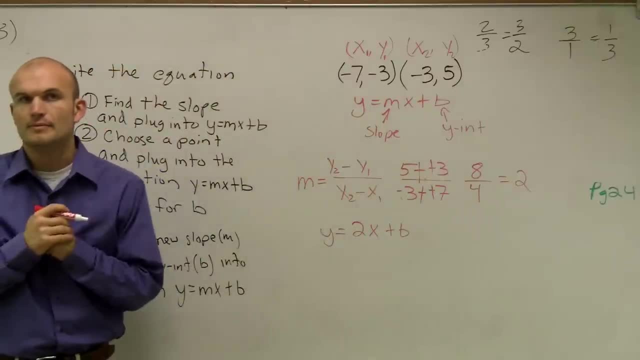 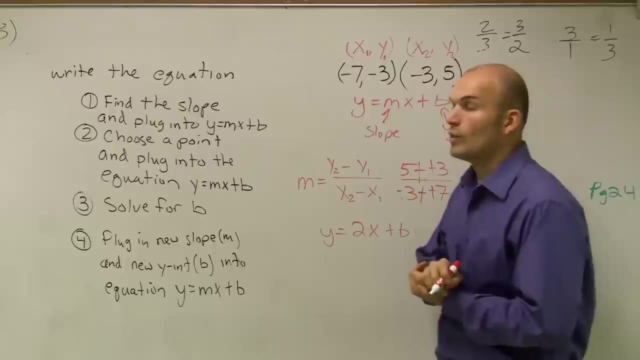 Because I'm saying I want 2 to represent my new slope. All right, So now I know what the slope is, but I don't know what the y-intercept is, And so it says: choose a point, Choose, Choose a point.